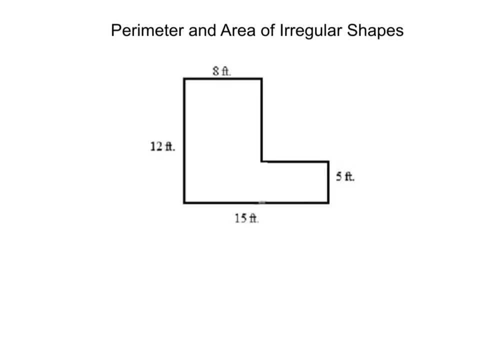 So we've covered finding the perimeter and area of basic shapes. but what if we've got an irregular or an odd looking shape, like we do here? First off, keep in mind perimeter and area have not changed. Perimeter is the distance around and area is the space that fills in the region. 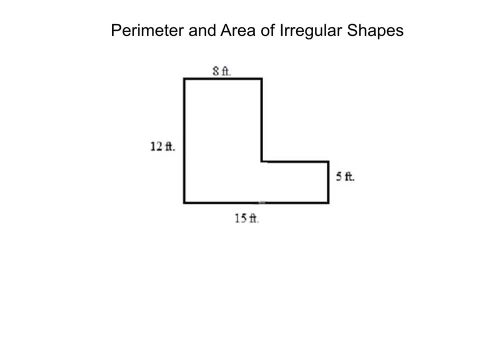 within the shape. The first thing I like to do in these is identify if I have any missing measurements Here. I do not have a distance or a length for this segment, nor this segment, So let's find those first. Let's go ahead and compare some of our side lengths and see if we can make. 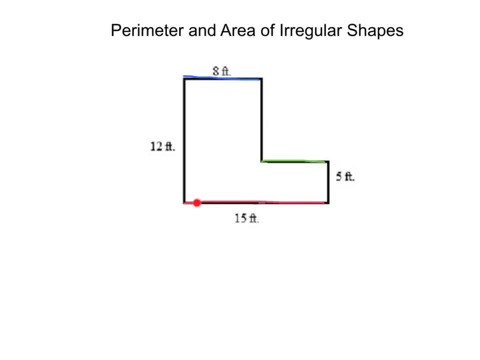 any progress. I see that this red segment here, the bottom segment, is a length of 15 feet. My blue segment up here is 8 feet and my missing segment I want to solve for in green is right here. Now, if we shift this green segment up, 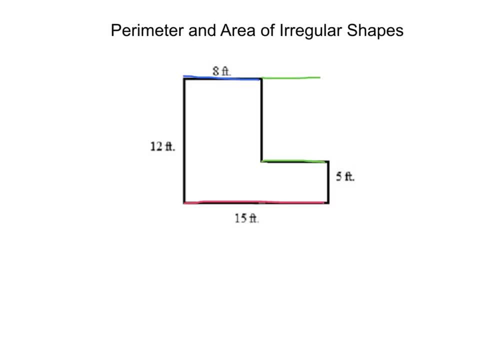 we can do that just because we're interested in its length only, We can see that the blue and green segment together should be the same length as this red segment that has a length of 15.. Knowing that, I can say, okay, well, if this is 8 feet, whatever my green segment length is. 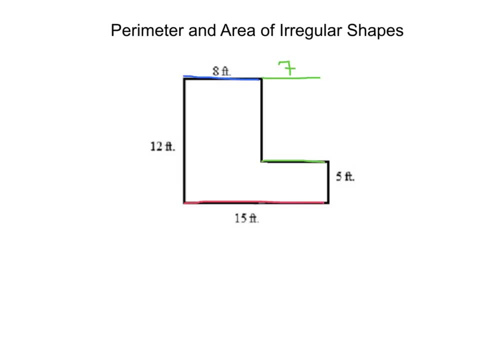 it's going to have to add to 15.. That tells me that this length has to be 7, because 8 plus 7 is 15.. You could find that just by seeing what number adds to 15. Or subtracting 8 from 15.. Either way, we found our missing length here. Let's see if we could find our 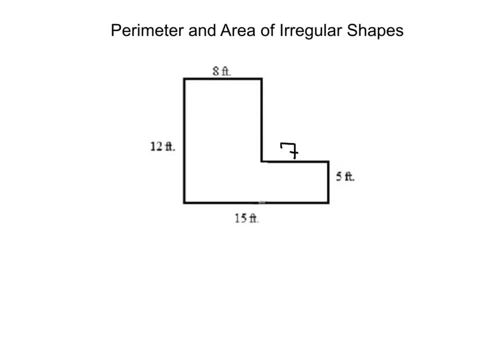 last missing segment by doing the same thing, only using the other line segments. to compare: In red I've got a length of 12 feet, In blue 5 feet And in green I'm going to go ahead and shift that over, just like we did before, And that's my missing length: 5 plus what is going to. 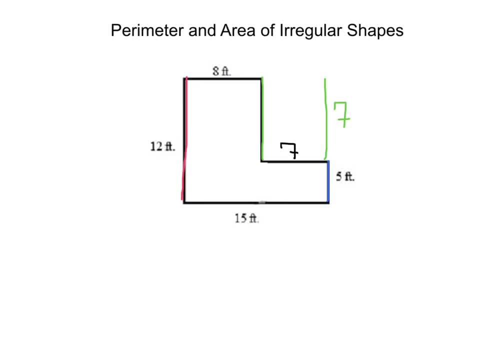 give me 12.. I can see that that green length is going to be 7 also, Now that we found our missing lengths, the perimeter is easy. We just need to add all of our sides around the shape. That's 15 plus 12 plus 8 plus 7 plus 7 plus 5, giving us a perimeter of 54 feet. Next we want to find the.